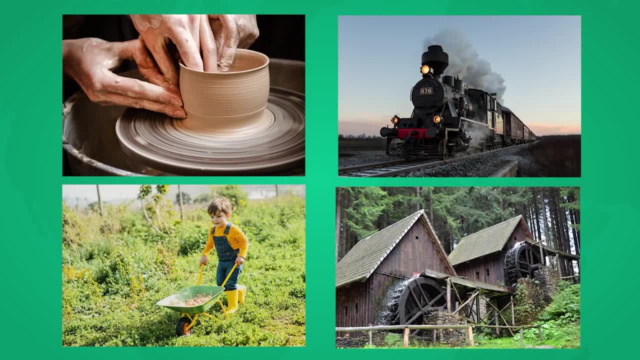 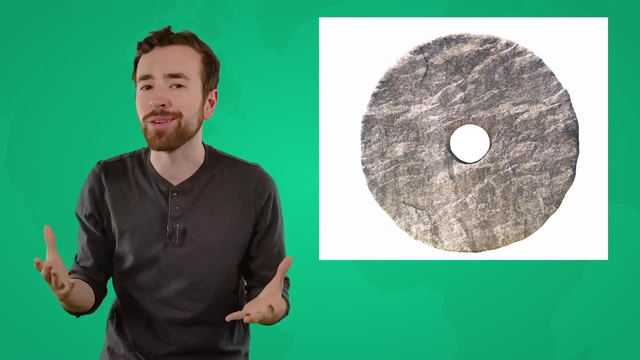 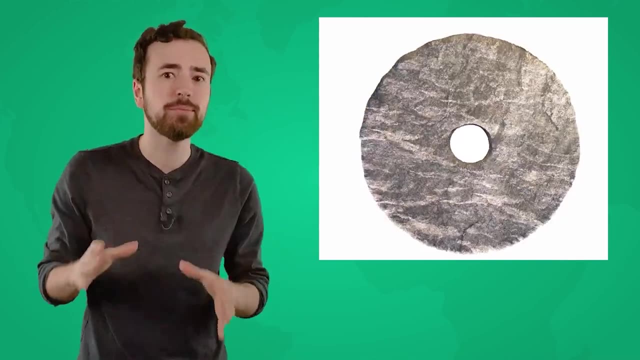 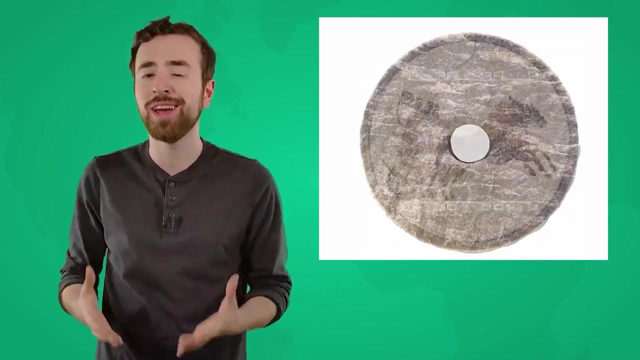 Can you figure out what that is? Time's up. Got your answer? Boom, You got it. It's the wheel, one of humanity's most revolutionary inventions. And guess what? This simple but game-changing invention is just one from a civilization that was an absolute powerhouse of ideas: Sumer. 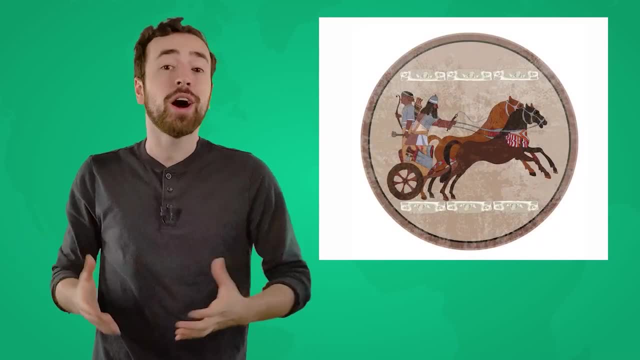 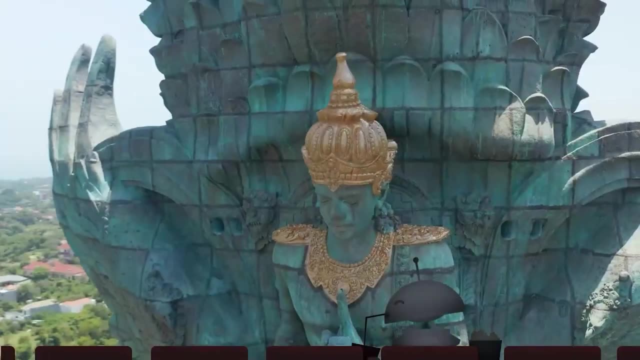 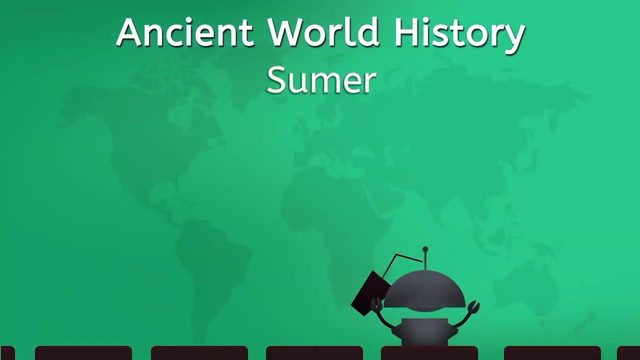 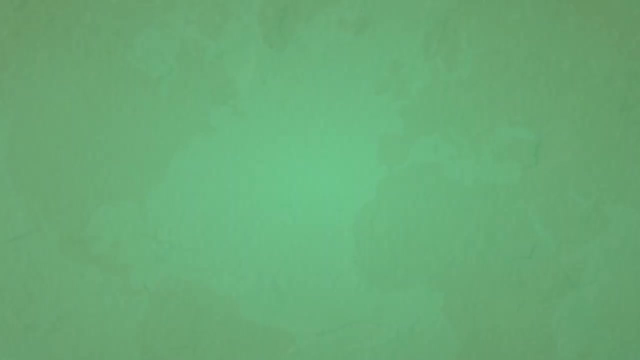 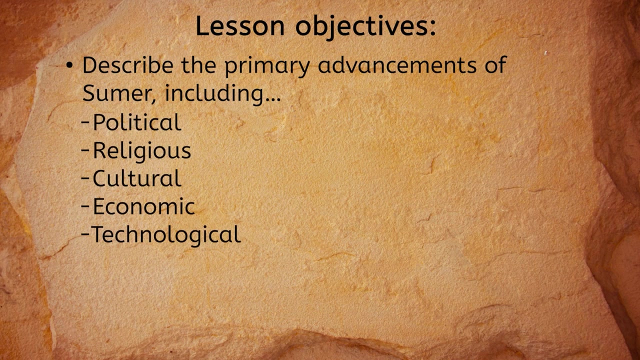 Now let's roll back in time and discover the wonders of this amazing place. Let's go. historians, Before we wheel out today's lesson, let's look at our objectives. We'll describe the primary advancements of Sumer, including their political, religious, cultural. 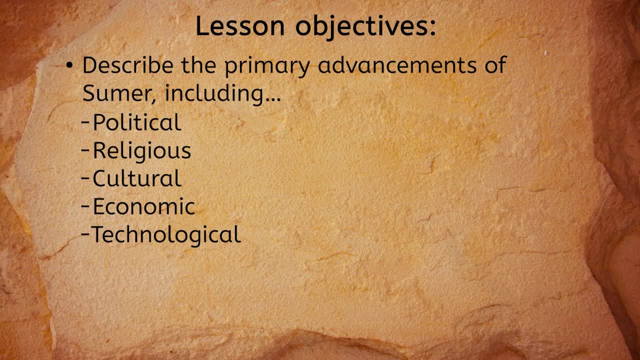 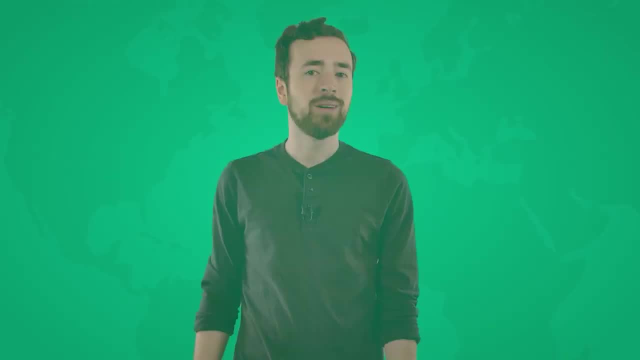 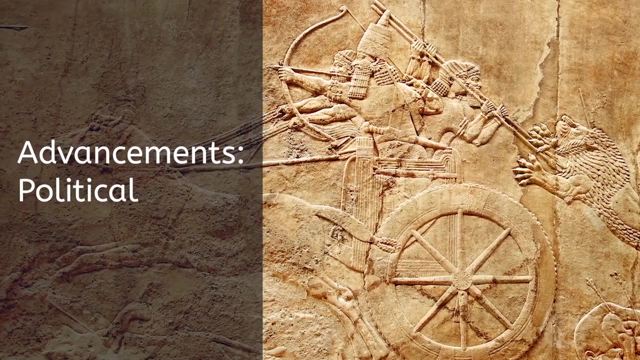 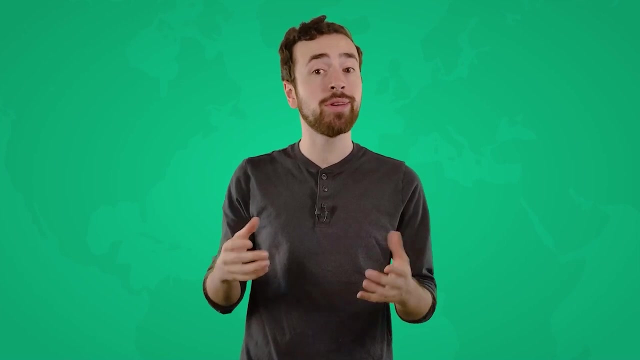 economic and technical advantages. We'll also look at their technological achievements And as we go, we'll explain how those advancements affected later civilizations. Are you ready, historians? Let's dig into the details of Sumerian society, starting with- you guessed it- government. 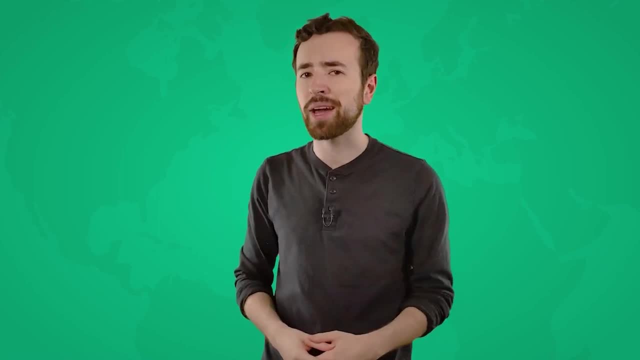 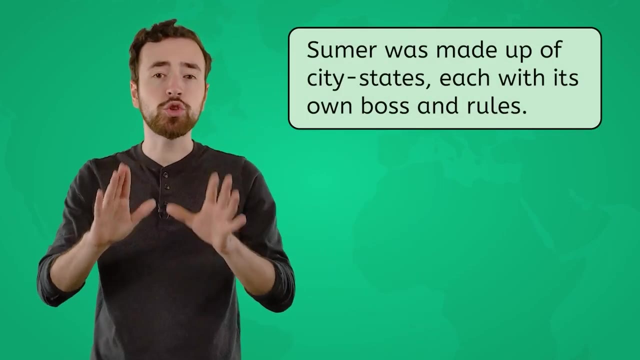 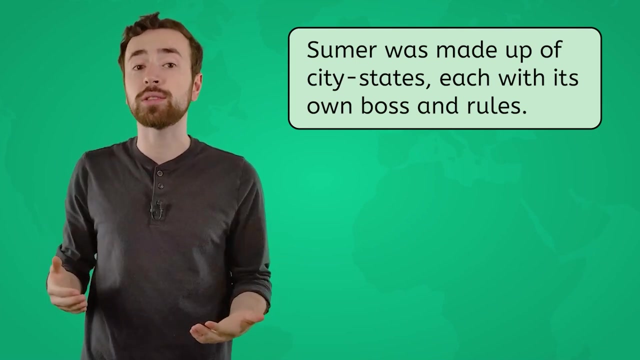 What kind of leaders and laws do you reckon they had back then in Sumer? Let's see if you're right. Picture this: Sumer was made up of a bunch of city-states, kind of like mini-countries, each with its own boss and rules. 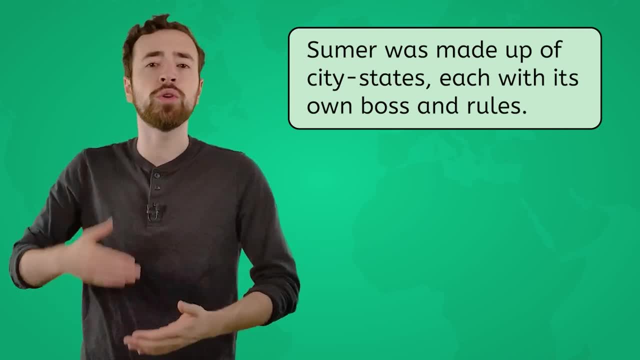 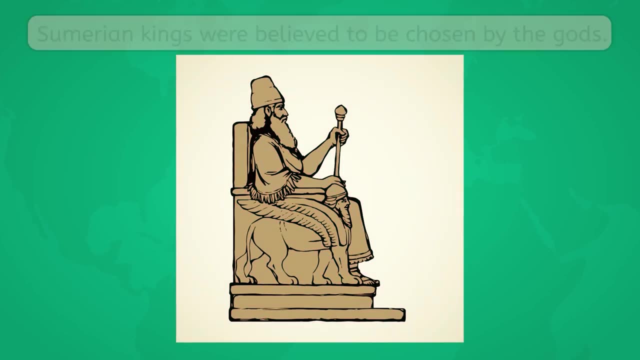 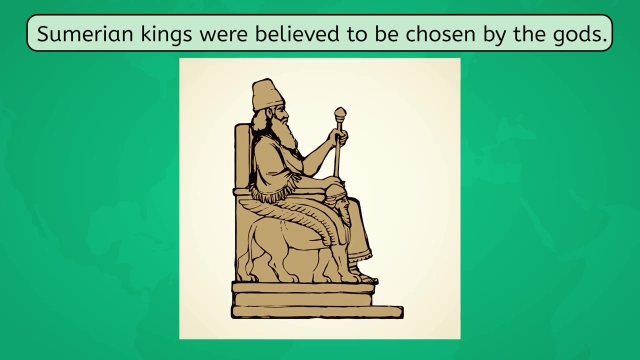 Imagine each city-state running its own show with its own laws, economy and soldiers. Cool right. And here's the kicker: These bosses, the kings, were believed to be hand-picked by the gods. This tied government and religion together. 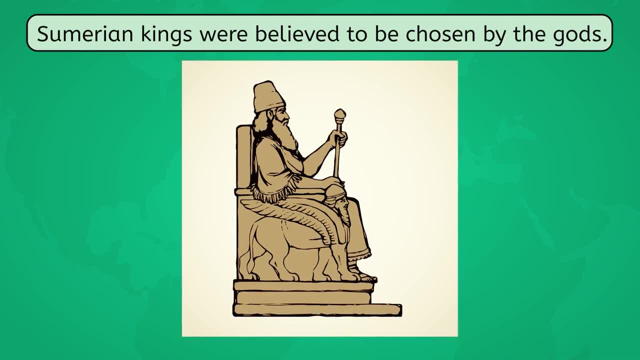 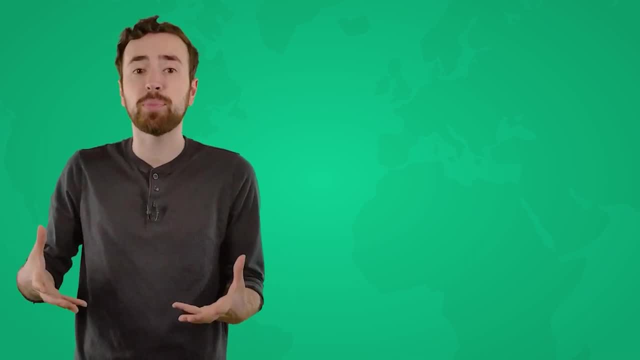 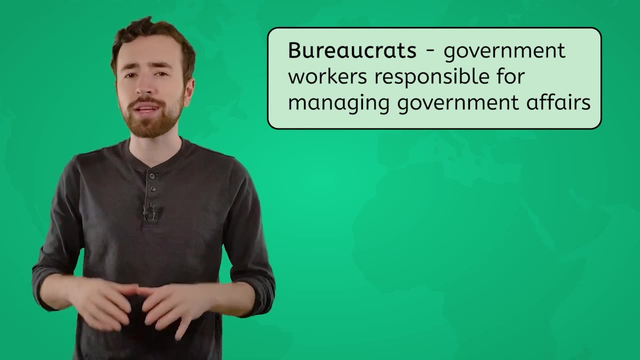 They would even have artwork and epic stories made, portraying them as god-like heroes. These kings ran the show, but they were helped by a big team of people called bureaucrats who did most of the work. These folks made sure everything in the city-state ran smoother than a chariot ride on a new Sumerian. 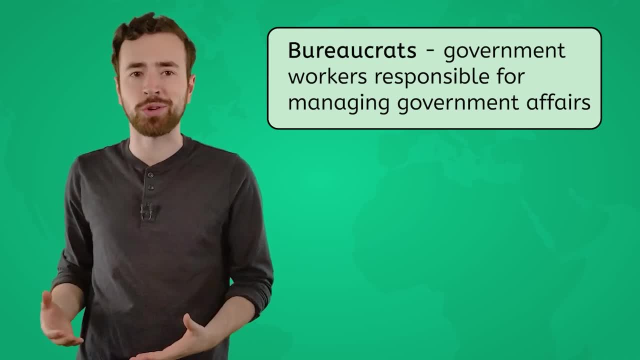 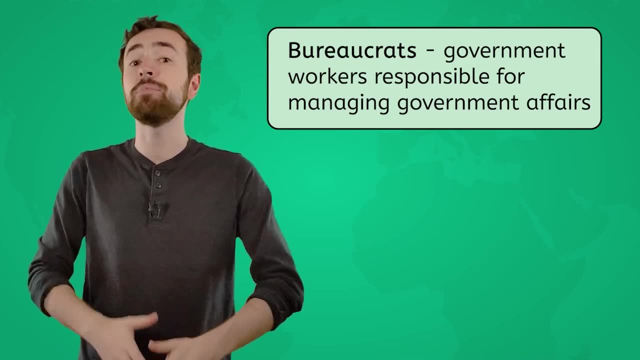 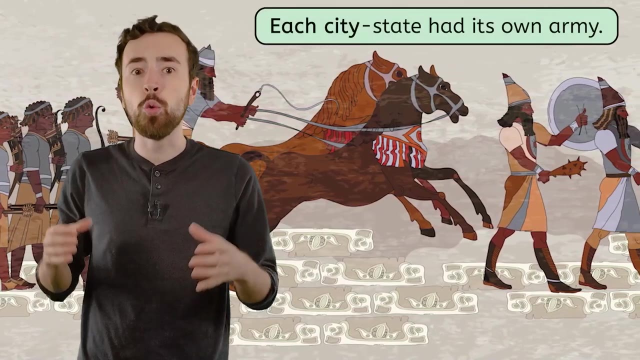 road. And these bureaucrats weren't just desk workers and managers. A bunch of them, trapped in the city-state, Traveled far and wide to talk to people in other city-states, trading goods and making peace treaties. But just in case, to keep the city safe, each city-state had its own army ready to defend. 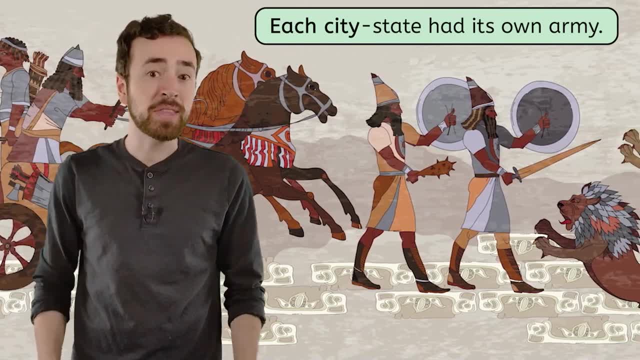 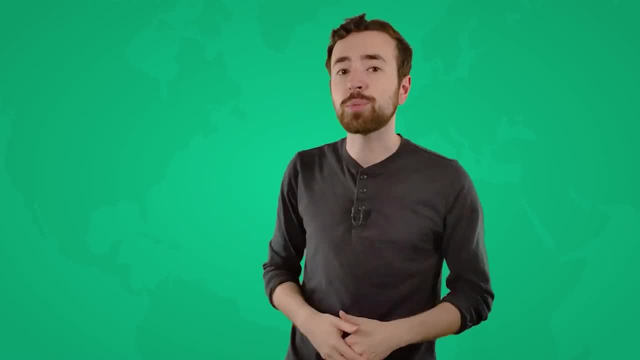 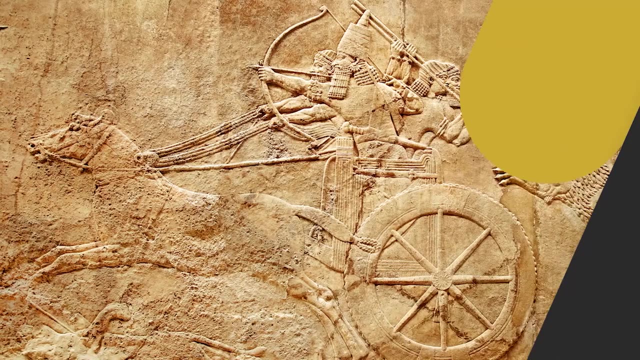 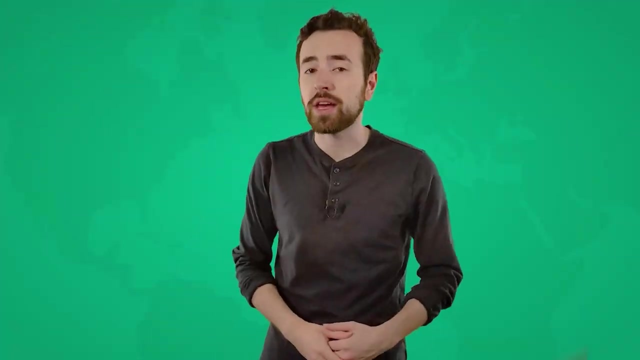 its home turf. Here's the best part. These ways of running things influenced other civilizations for centuries. Many of Sumer's ideas on government, even though they've been tweaked, are still in use today. Sumerian Kings: We said earlier that Sumerian kings were also religious leaders and were helped by priests. 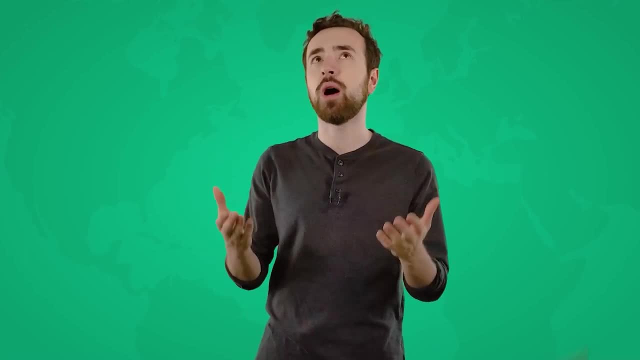 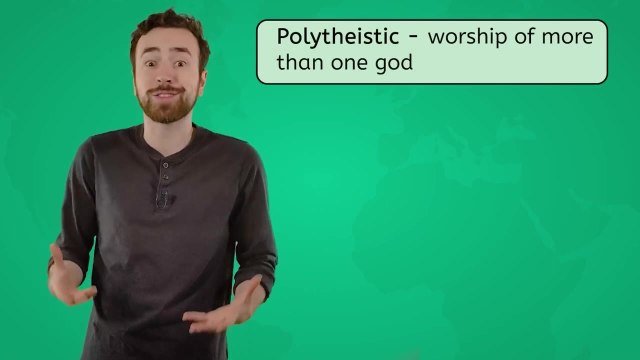 Together they led religious rituals and ceremonies to honor the gods. Now imagine having not just one or even two, but a whole bunch of gods to pray to. That's what being polytheistic means: The worship of more than one god. 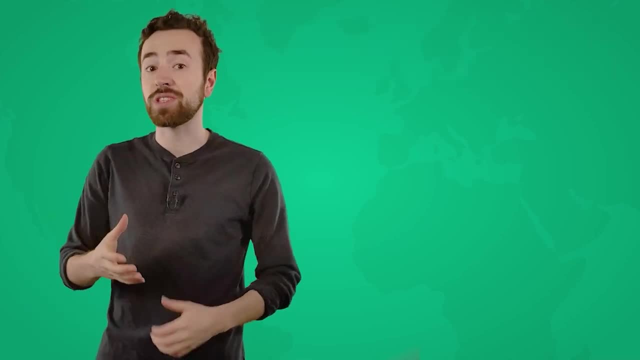 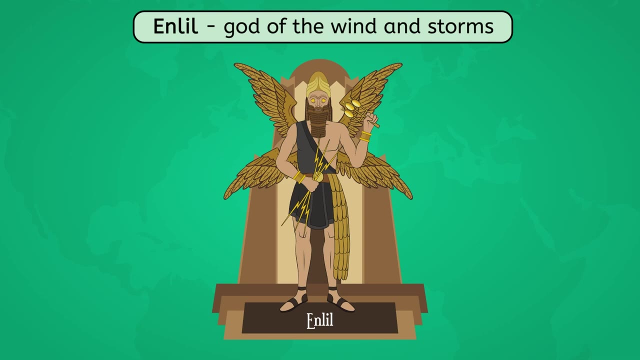 And most Sumerian gods represented forces of nature. Take Enlil, for example. He was in charge of the wind and storms. He also controlled the rain, which makes him pretty important if you're a farmer hoping for a good crop. 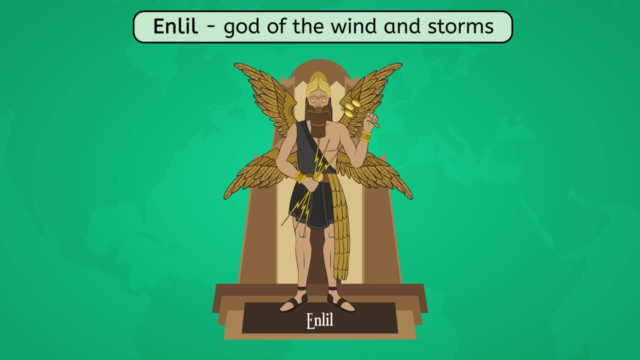 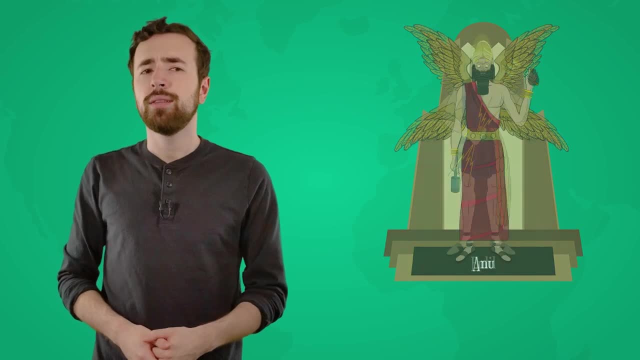 Want to learn more about Sumerian gods, Then be sure to check out the PDF. Since these gods ruled forces which were important in the lives of Sumerians, they were usually included in prayers for nice weather and peace. They were also included in the religious rituals of the gods. 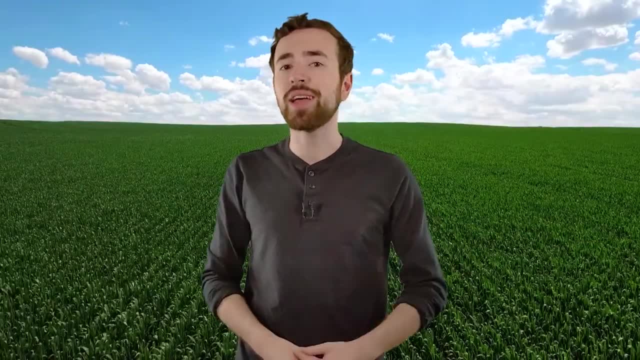 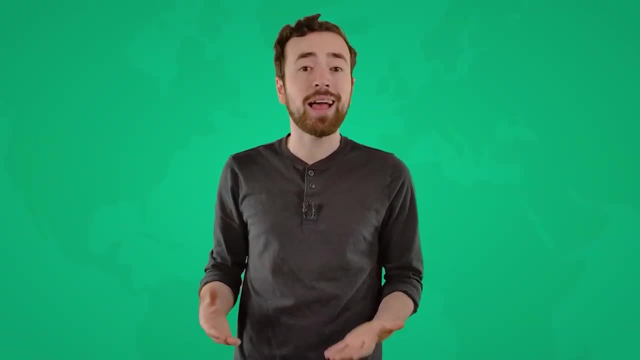 Honoring the gods that controlled their crops made people feel like they were in control of their own destiny. Polytheism wasn't just a Mesopotamian thing either. Having many gods was the norm for most, but not all, early civilizations. 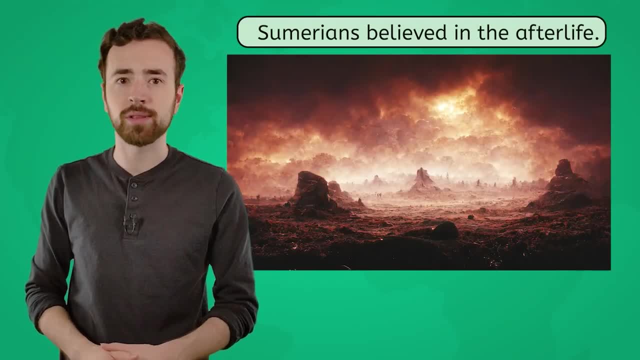 Sumerians also believed in an afterlife, But to them it was a dark and gloomy place which made life on Earth even more important. Sumerians also believed in the afterlife, But to them it was a dark and gloomy place which made life on Earth even more important. Sumerians also believed in the afterlife, But to them it was a dark and gloomy place which made life more important. Sumerians also believed in the afterlife, But to them it was a dark and gloomy place which made life more important. 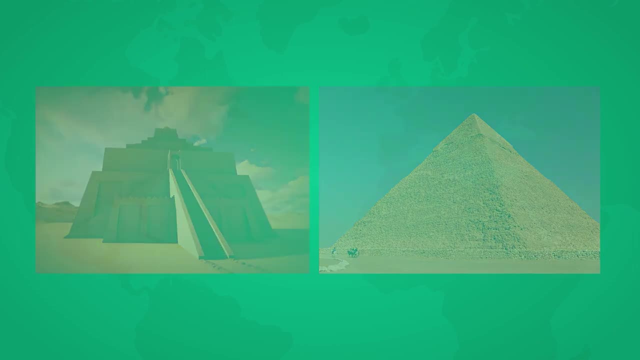 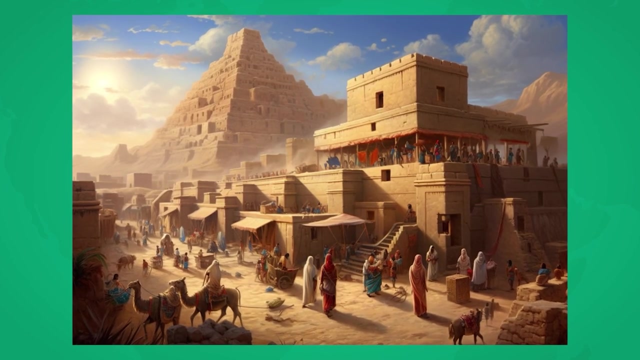 Wow, Where did they worship these gods guys? At ziggurats. These were giant temples that were the heart of the town. Kind of looks a little familiar. huh, Picture this: a huge building where people went to pray. Around it they could also meet friends and even do a little shopping. 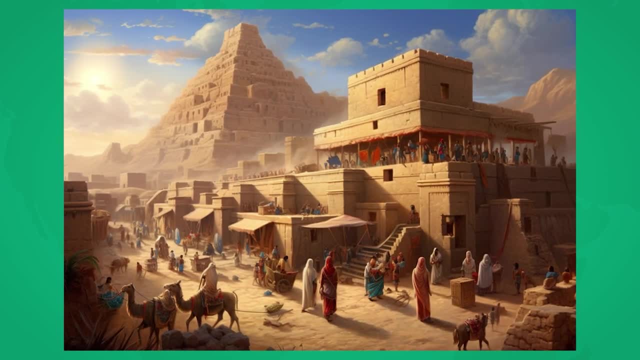 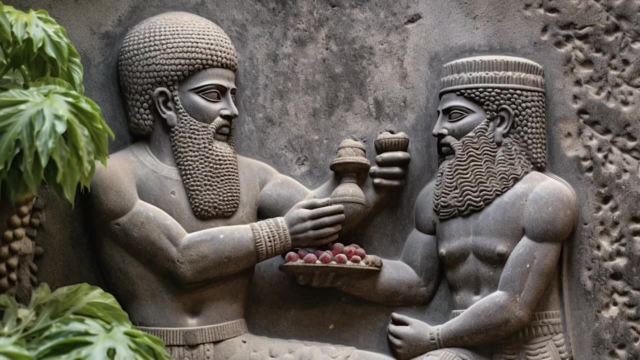 Kind of like the ancient version of a mall. This is way bigger than the main jinan that we saw during the non-CEO banner era. in showing their gods some love by giving them presents- These weren't like birthday gifts, though. They offered animals food and drinks to win their god's blessing. 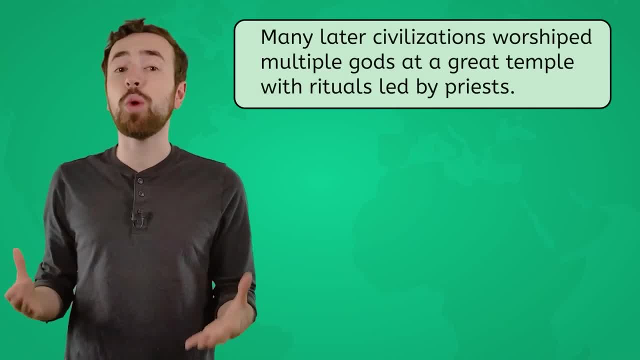 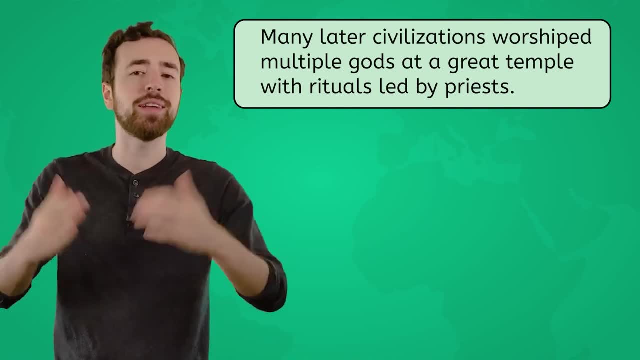 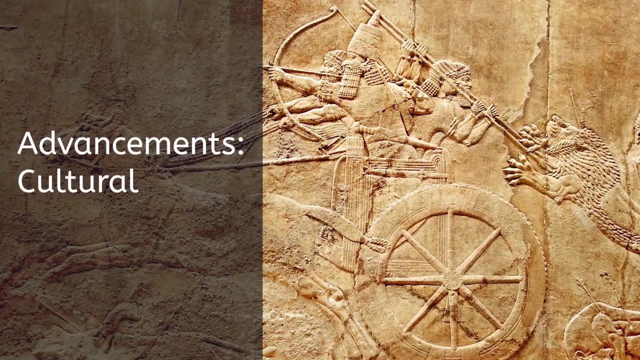 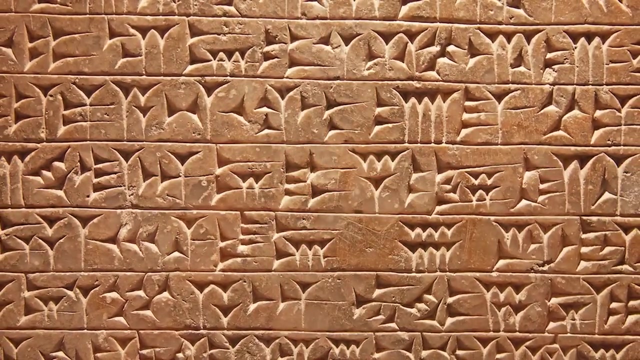 And here's a neat fact to wrap things up: The Sumerians' way of worship influenced many later civilizations who also prayed to multiple gods at grand temples led by priests. So you could say the Sumerians were trendsetters. One of the biggest cultural achievements was cuneiform. 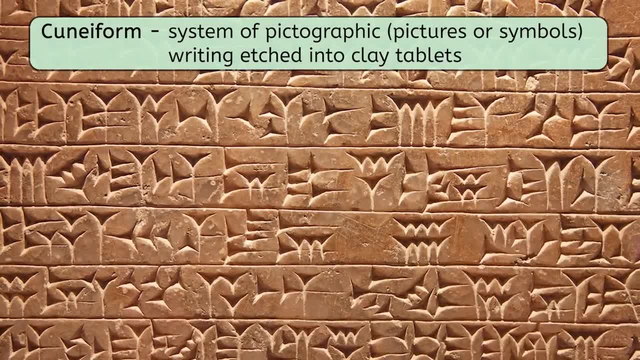 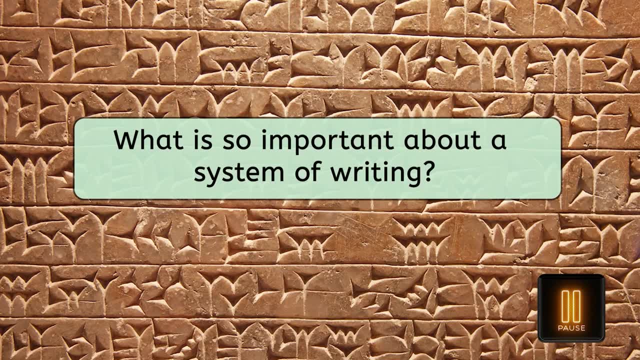 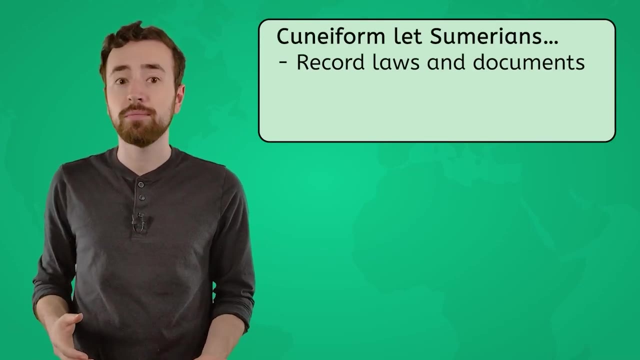 a system of writing where little pictures were etched into clay tablets. Here's a question for you: What is so important about a system of writing? Pause here to respond. Among other things, cuneiform. let Sumerians write down their laws and government documents. 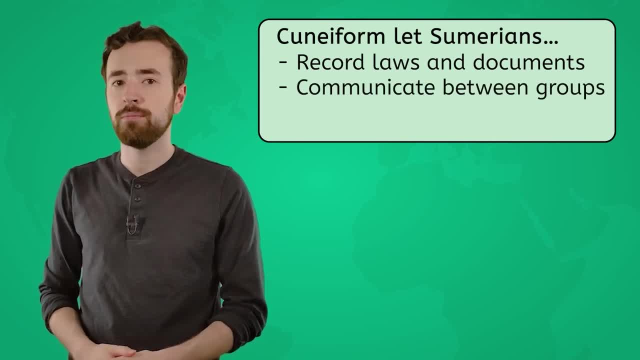 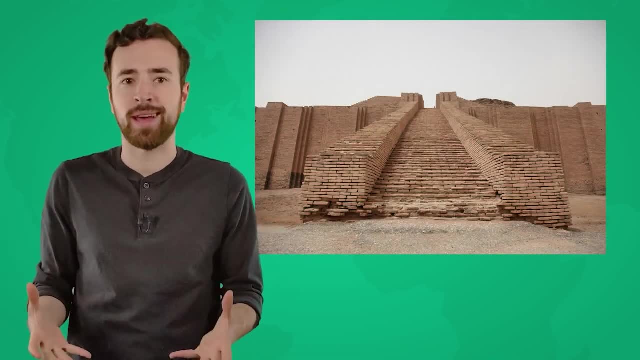 and made it easier to communicate between different groups. They could write down their history too. I mean, just imagine trying to build a ziggurat without a plan written down. How would thousands of workers know what to do or where to go? 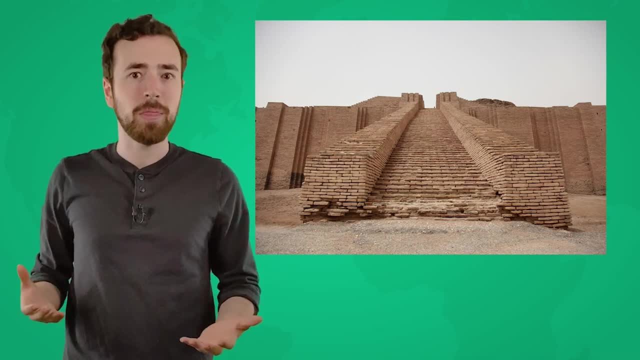 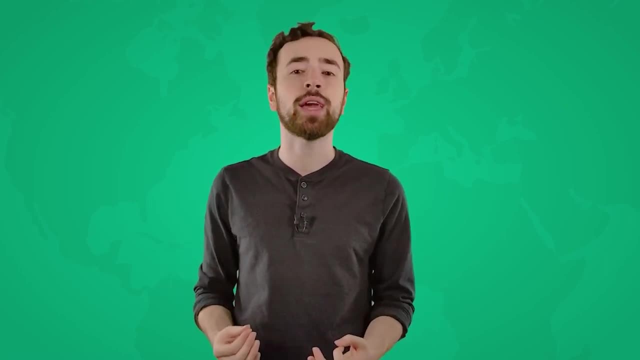 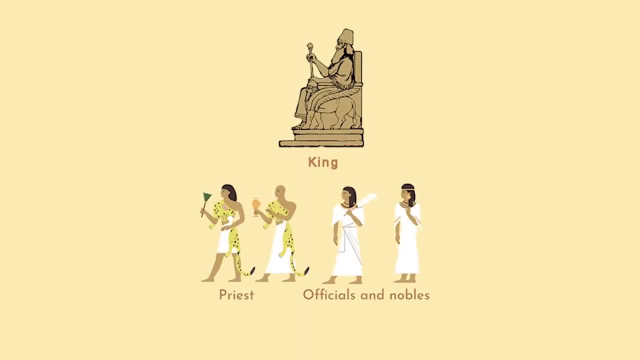 How would the people in charge stay organized, Even though several city-states had their own spoken language? cuneiform was a consistent form of communication, but it was also a form of communication across the land. Imagine people being grouped by their jobs. That's what happened in Sumer. 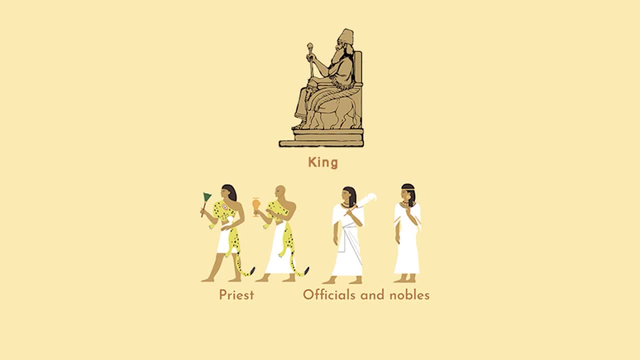 A social structure based on jobs developed in the region. At the top were the ruling elite, which was made up of kings, priests, nobles and high-ranking officials. This group is the one that was in charge of everything in Sumer. 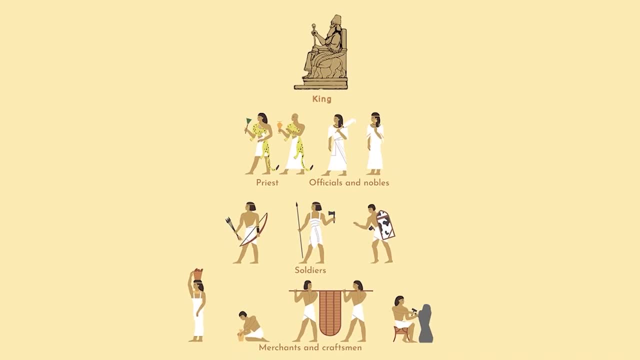 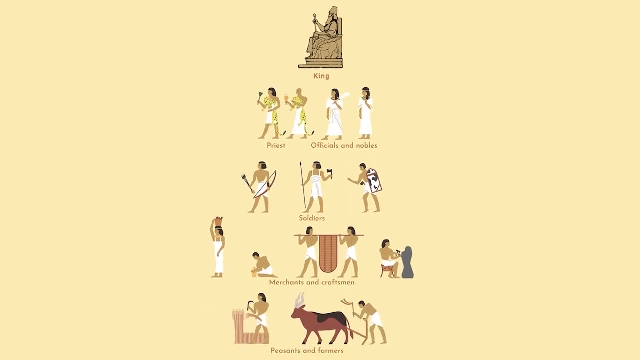 Below them were commoners. These folks were divided into several levels, including soldiers, merchants and skilled workers, And below them were farmers. These people protected the city, owned and operated markets, made things such as pottery and jewelry, and provided food to everyone. 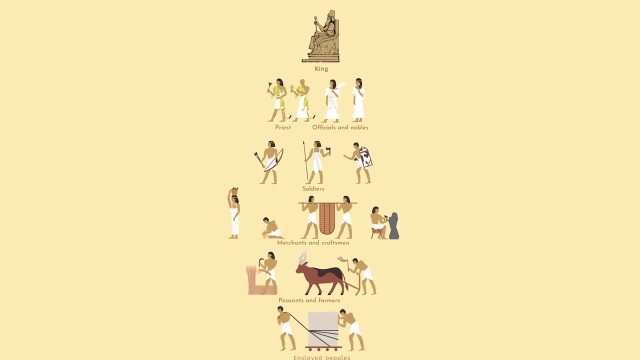 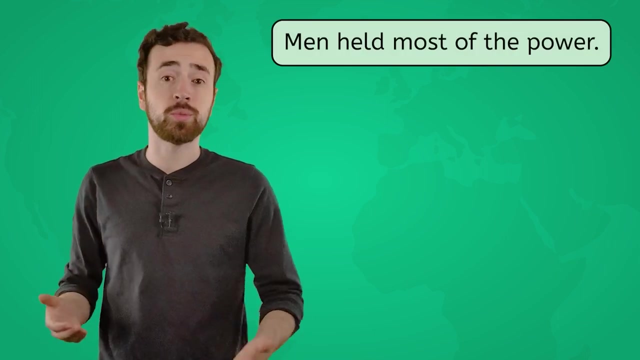 Important jobs for sure. And at the very bottom were enslaved peoples who were usually prisoners of war or people who had been sold into slavery to pay off debts. Gender played a big role in Sumerian society. Med had most of all the most important role in Sumerian society. 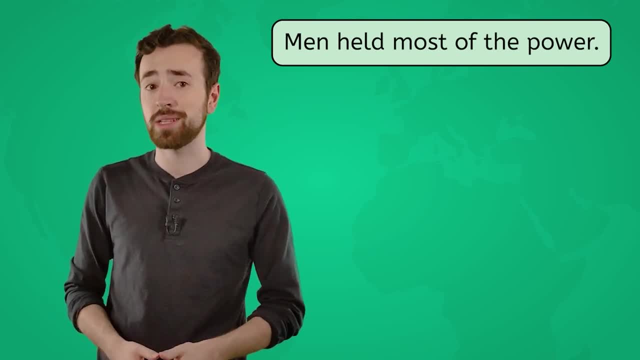 Med had most of all the most important role in Sumerian society. Med had most of all the most important role in Sumerian society. Most of the power and women were usually limited to supporting their families at home. This was common for future civilizations too. Sumer served as a model civilization for others, as writing was later created in other civilizations as a way to communicate, And social classes like those in Sumer became the norm. I mean, it worked well for Sumer. 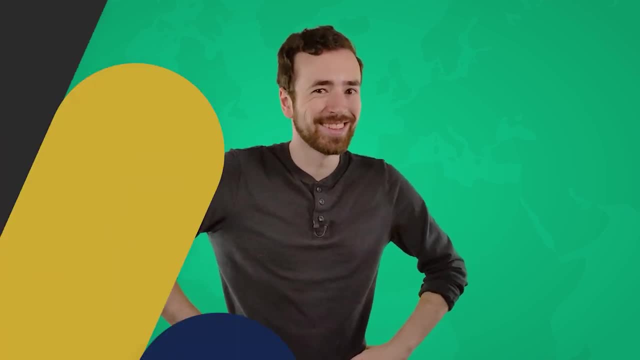 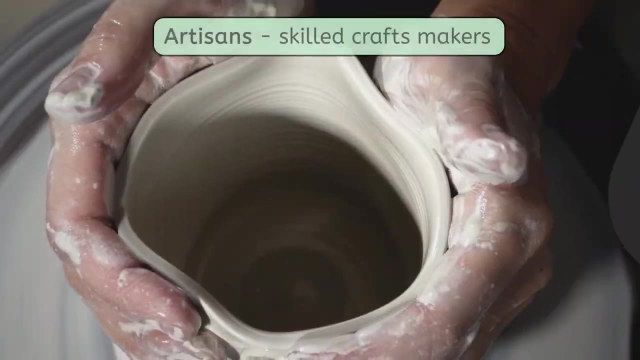 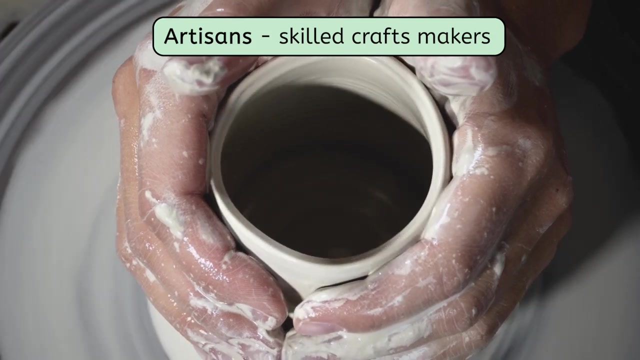 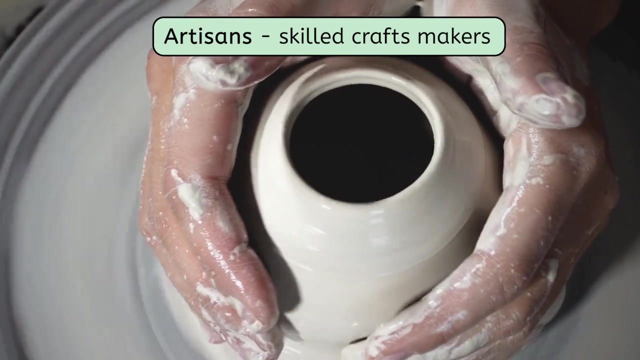 Why reinvent the wheel right? Specialization led to all sorts of jobs, like you saw in the social classes, as people tried to make their lives better based on their skills. Those jobs also included fishermen, scribes and artisans, or skilled crafts makers like potters. 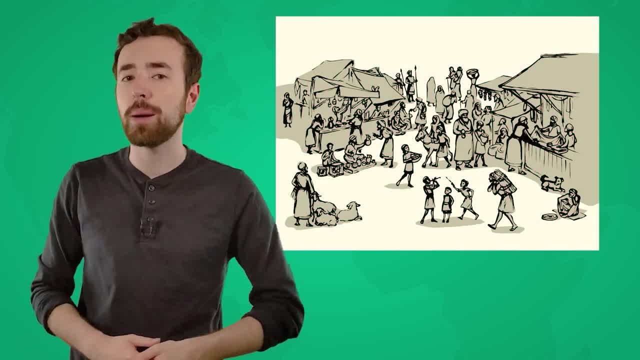 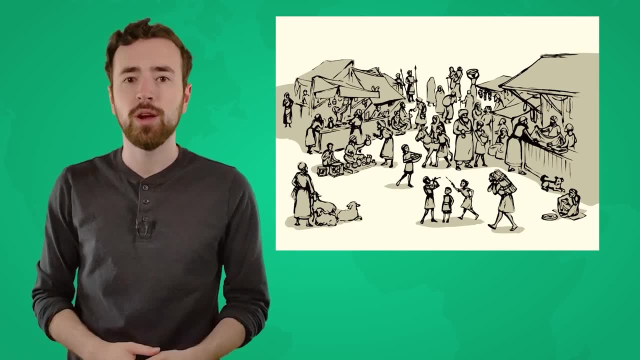 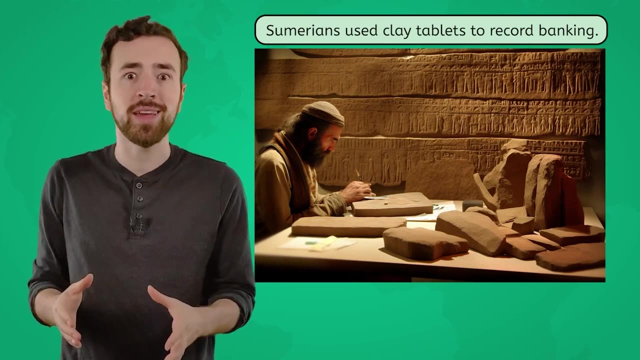 Sumer had a massive trade network that allowed them to swap goods with other civilizations too. They traded things. they had a lot of, like wheat and precious metals, for goods that were more scarce, like timber. Sumerians were the first people to create a system of banking. 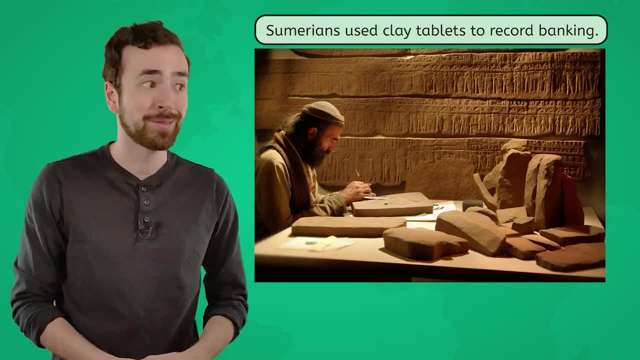 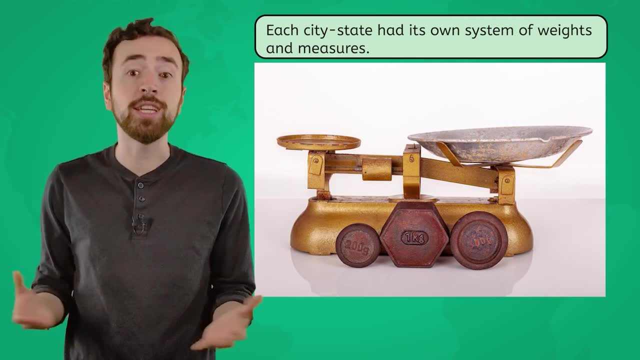 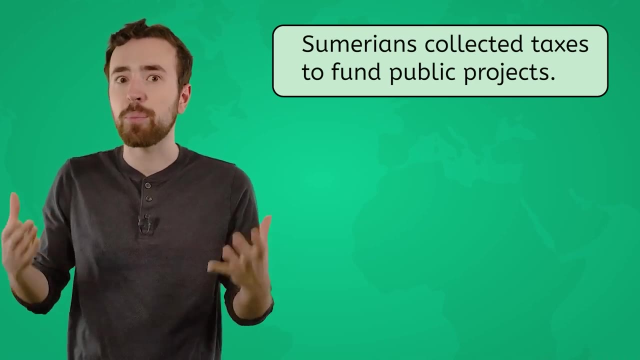 using clay tablets to record the transactions- Cool huh. They also used weights and measures to make sure trade was fair, but each city-state had its own system. Sumerians collected taxes from people, then used the money to pay for public projects. 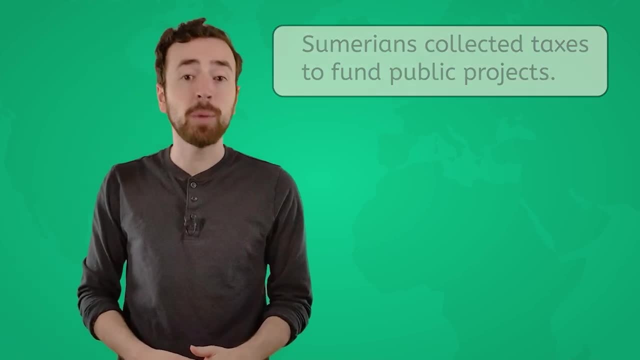 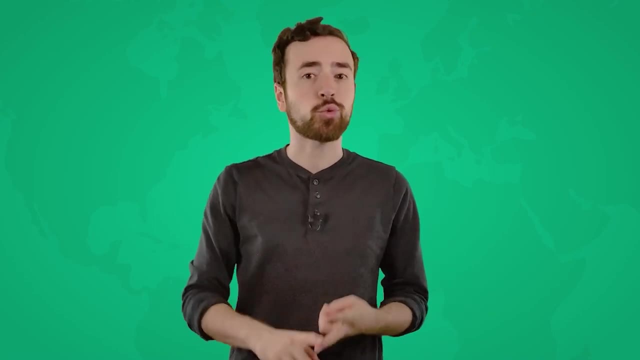 such as irrigation systems and ziggurats. A bunch of extra money from Sumerians was then used to make money for the people of Sumer. Sumerian economic advancements from Sumer were later copied by other civilizations: Specialization, trade, banking, taxes. 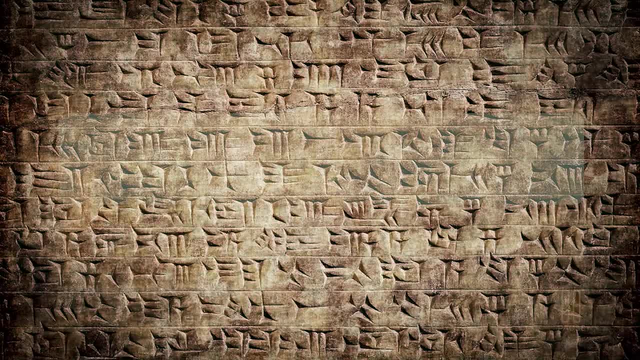 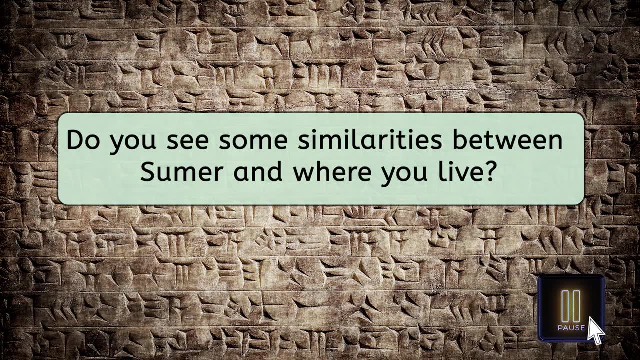 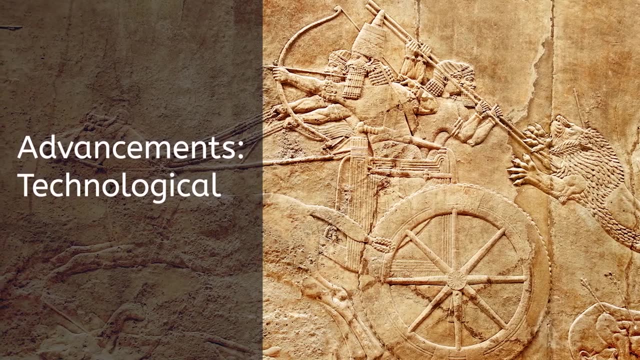 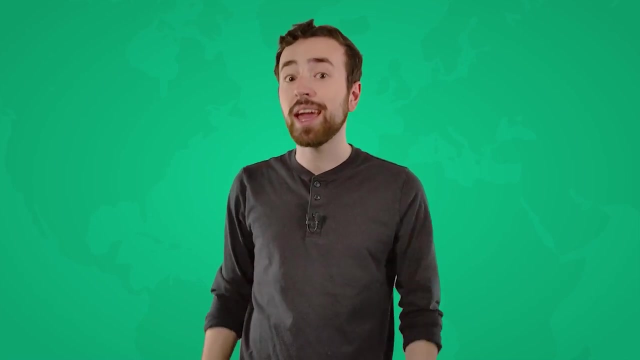 Just be careful asking your parents about that last one. Hey, so far do you see some similarities between Sumer and where you live? Take a moment to jot a few down. Some of the biggest developments in Sumer involved technology and new inventions. 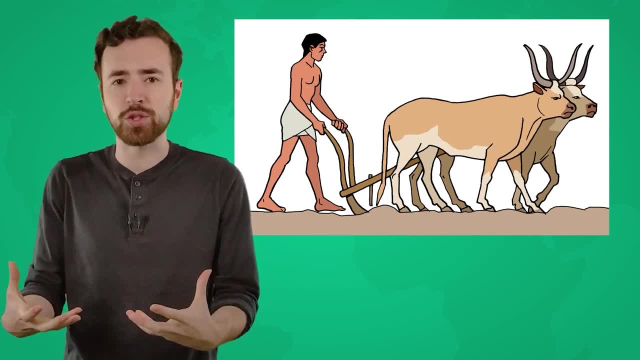 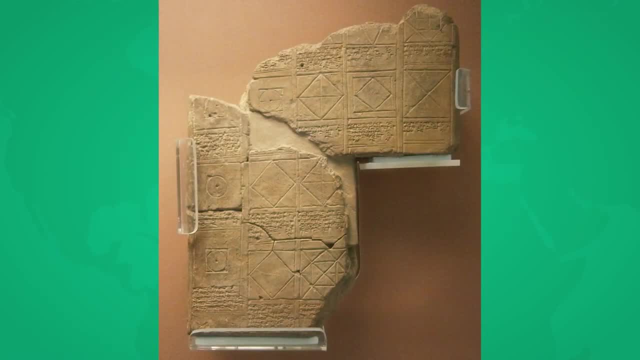 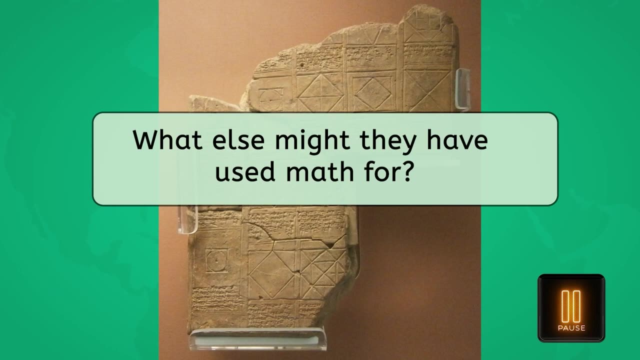 One that helped farmers was the plow, which broke up the soil and made planting crops much easier. Advances in math were important for a bunch of reasons. Now, you've already heard that Sumerians used math for both banking and measurements. What else might they have used math for? 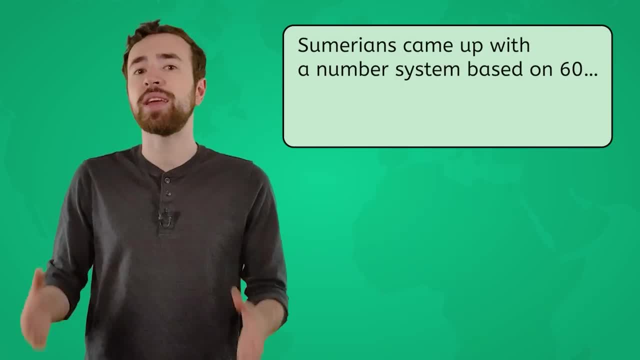 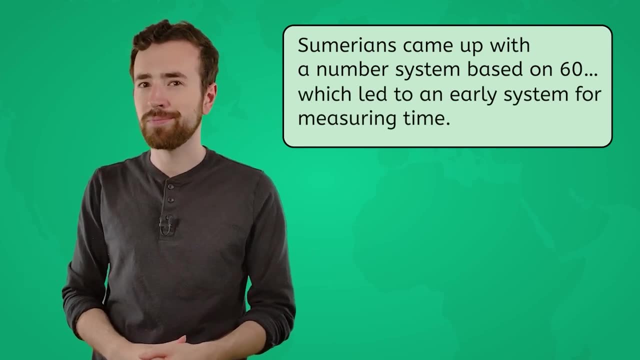 Well, the Sumerians came up with a number system based on 60. This helped with an early system for measuring time. Think about it: 60 minutes in an hour, 60 seconds in a minute. Yeah, Sumer did that. 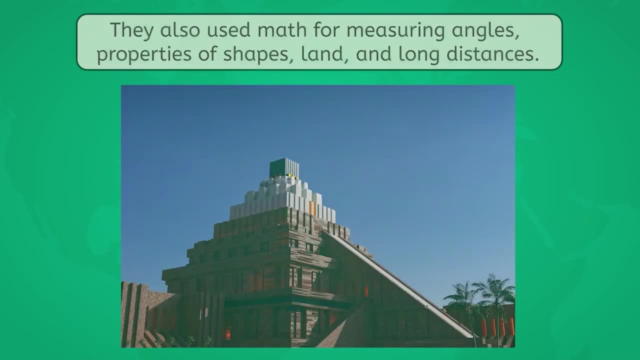 And they used math for measuring angles. Sumerians were able to measure the properties of different shapes, which really helped them with architecture and building things. They also used their math to measure the size of buildings. Sumerians used their math to measure the size of buildings. 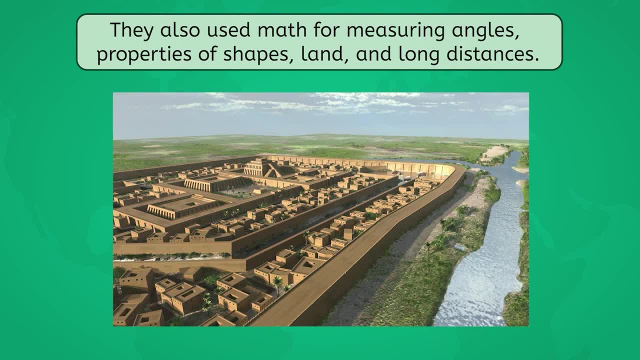 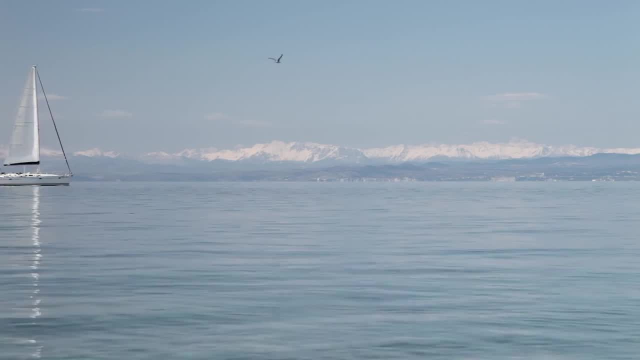 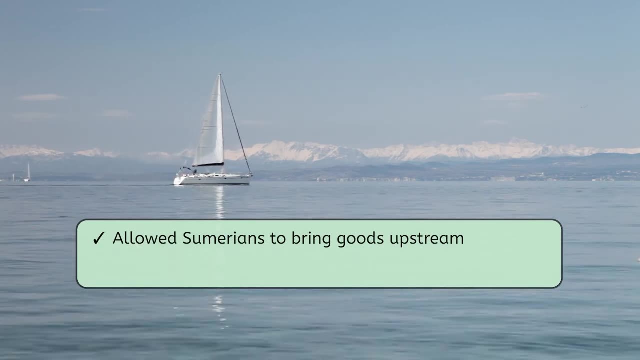 They also used their math skills to measure land and long distances. That made travel and trade a lot better. And here's one that changed transportation and trade forever: That sailboat. It let them easily move goods upstream, which before had been really tough. 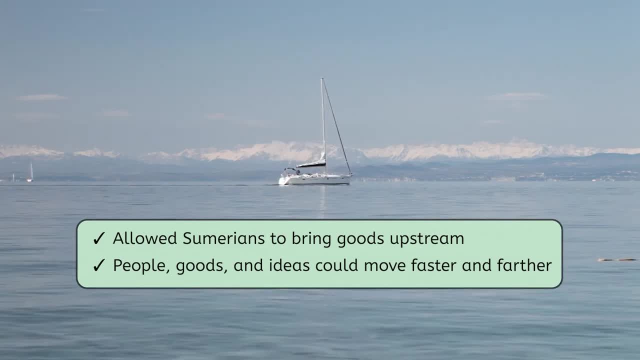 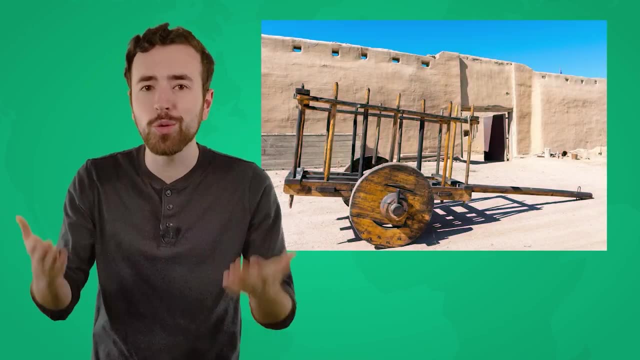 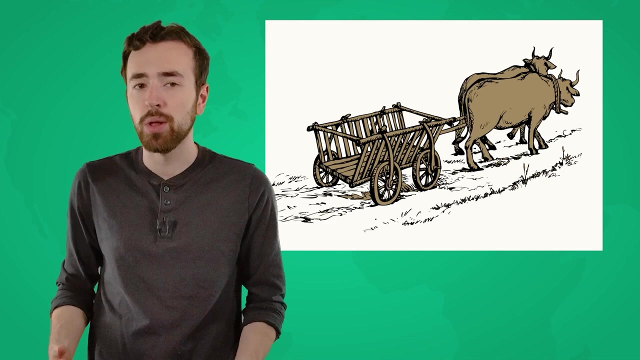 And it meant people, goods and ideas can move faster and farther than ever before. And I'm sure you remember that the wheel was invented by Sumer. It was used on carts and wagons pulled by animals or sometimes even people. 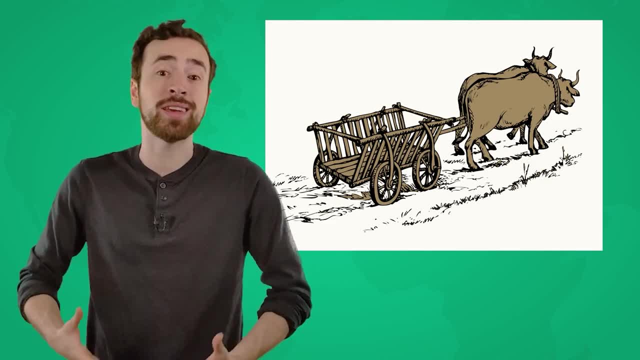 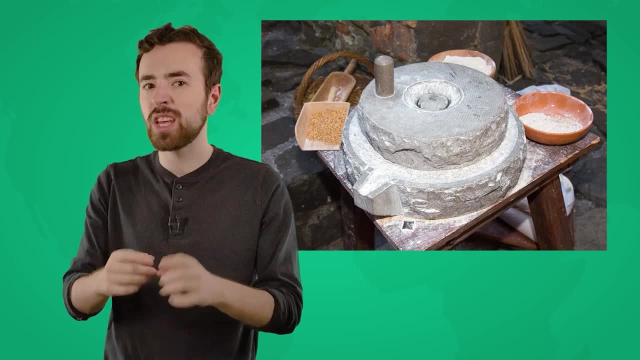 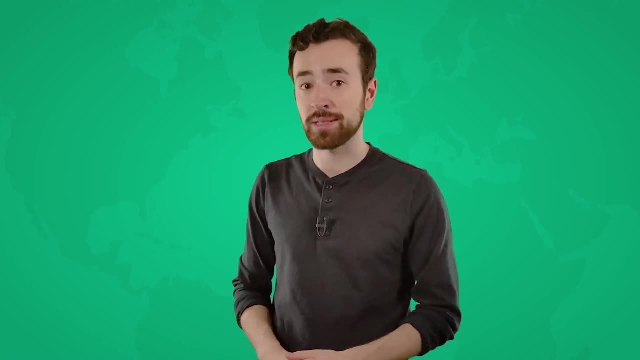 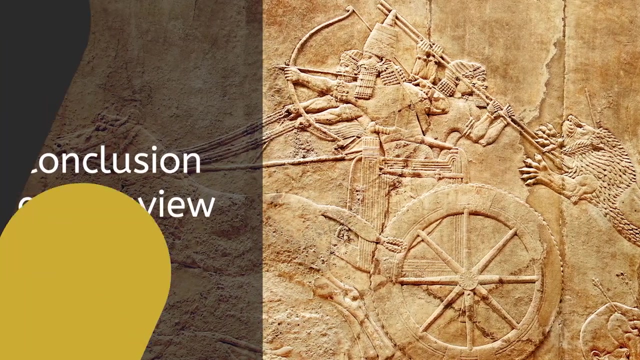 to move stuff a whole lot more than people could carry in their arms. They used pottery wheels to make clay pots and made mills and used millstones to grind grain into flour. All of these were used and improved upon by later civilizations. Now, keep in mind: all these things didn't happen overnight. 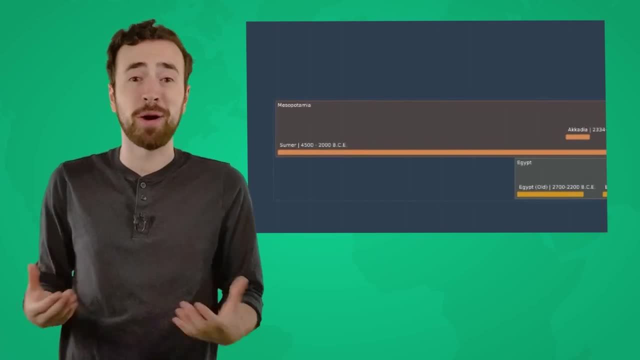 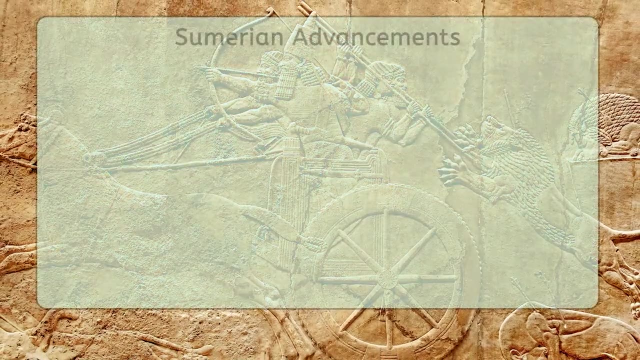 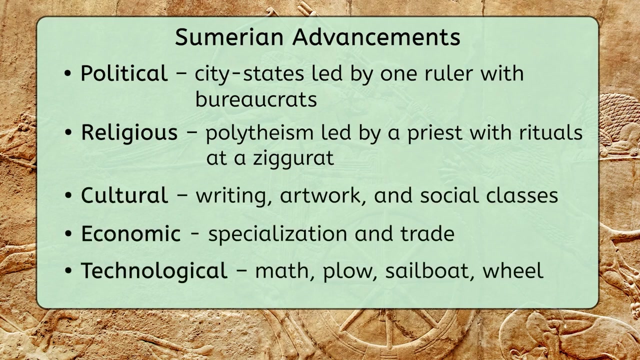 It took hundreds and hundreds of years for Sumer to come up with all these things, But good thing they did. These were huge ideas and inventions, not just in Sumer but for later civilizations all around the world. These ideas and others were copied and modified by people for centuries. 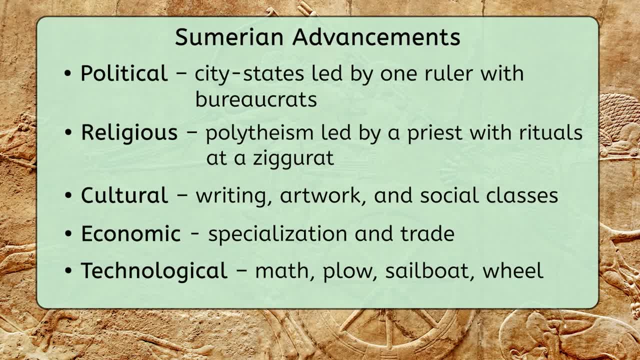 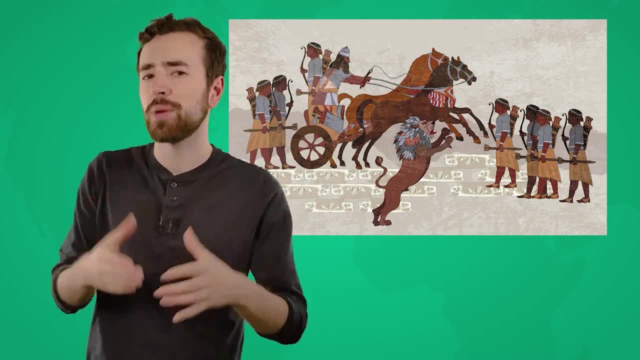 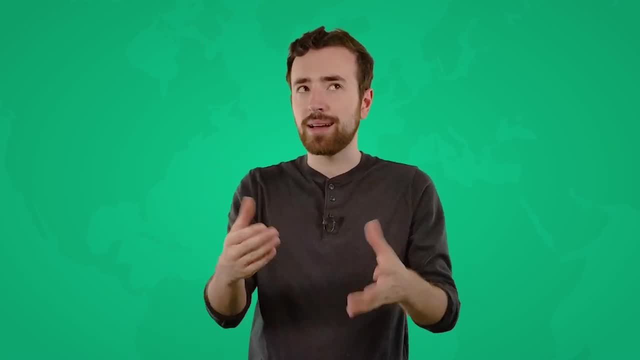 The Second World War. Next time we'll check out another civilization in Mesopotamia that used the Sumerians' ideas and inventions and then added a bunch of their own. Until then, historians keep uncovering the past and looking to the future. 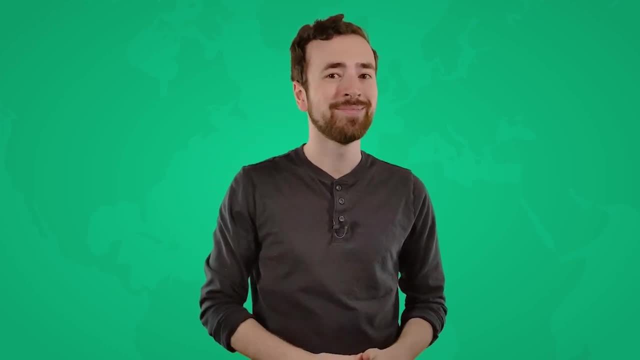 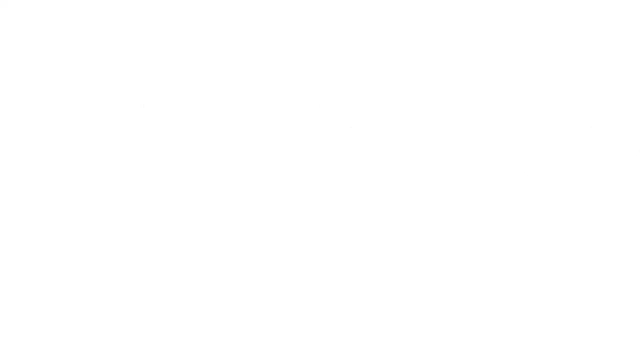 And remember to always be clever. Subtitles by Subtitle Workshop.